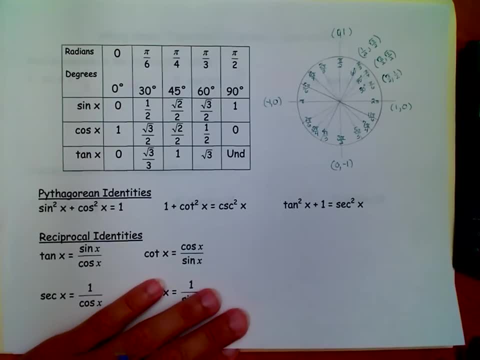 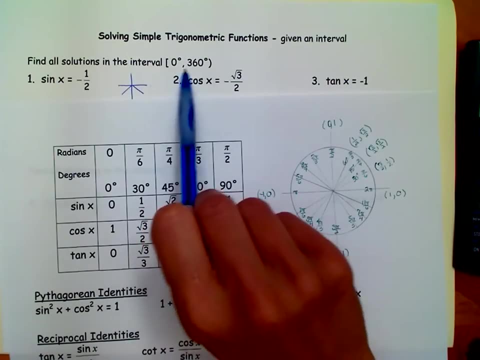 If you have not memorized that, then that's when you need this handy dandy little chart. Sine is one half at 30 degrees or in radians pi over six, But since it says here is 0 to 360.. We're going to use that 30 degree. 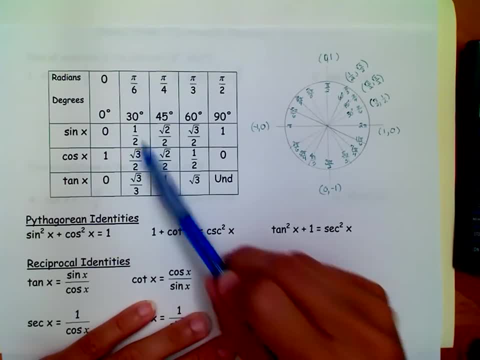 So, although it's one half at 30 degrees, I need to know where it's negative one half. Well, that would be again in these two quadrants. So I know that I'm 30 degrees down. That means this is the reference angle. 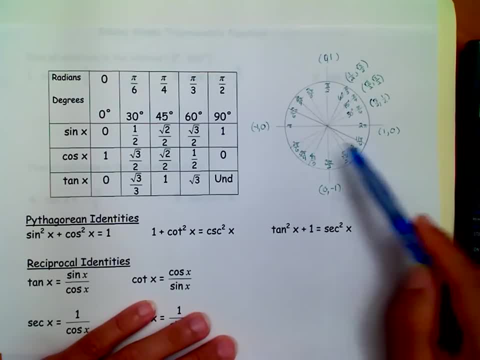 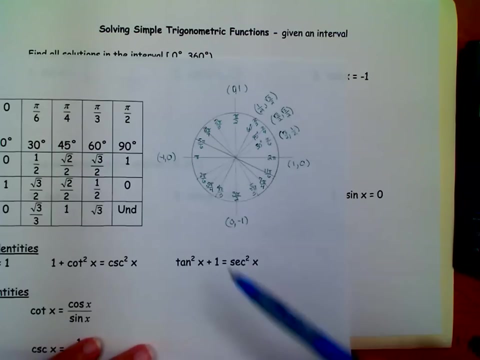 I'm 30 degrees down from the x-axis, So this is 180 degrees. So 30 degrees down would be 150.. This is 360.. So 30 degrees down would be 330.. Did I just say 150?? Okay, 30 degrees down. 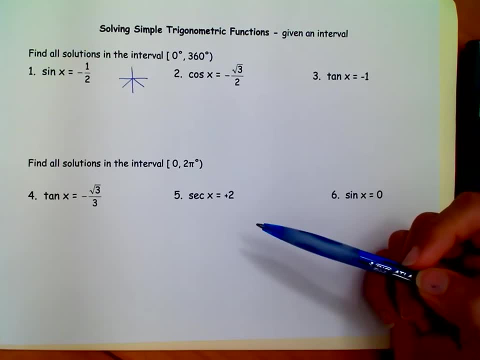 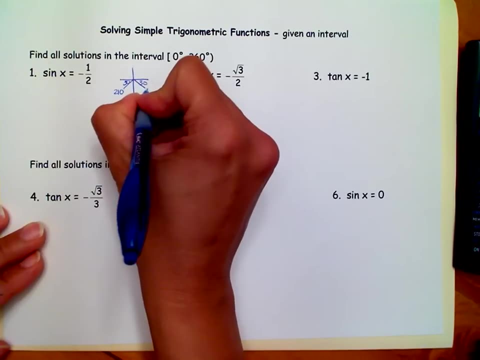 I'm not subtracting. That would be up 30 degrees, down is not 150. It's 210. So since I know that these are 30, then I know that this is going to be 210 and 330.. So those are my answers of where sine is negative one half. 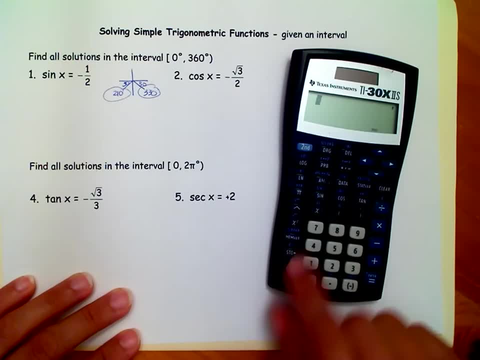 And if you're not sure, you could always just get out your calculator and say sine of 210. And that's negative a half. I had made that mistake and then checked If I had said 150, then we would have seen that it was positive one half and known that I had done something wrong. 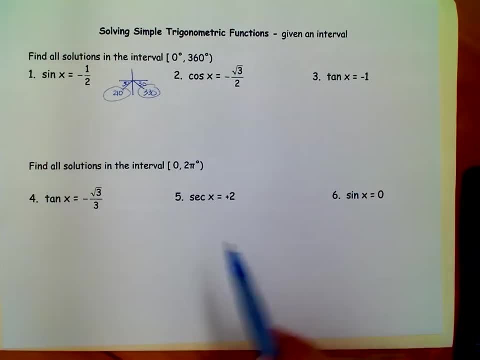 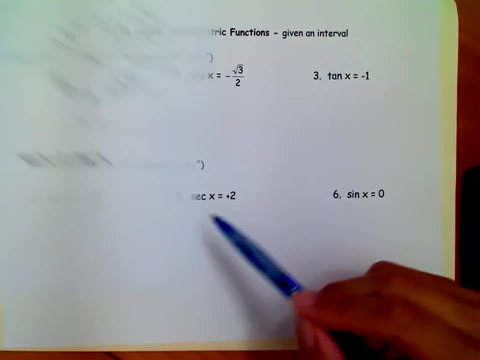 Okay, the next one. So cosine, When is cosine squared over 3, over 2?? That's the first thing we figure out. It's at 30 degrees as well. So we know that it's at 30 degrees And cosine is negative because cosine is x. 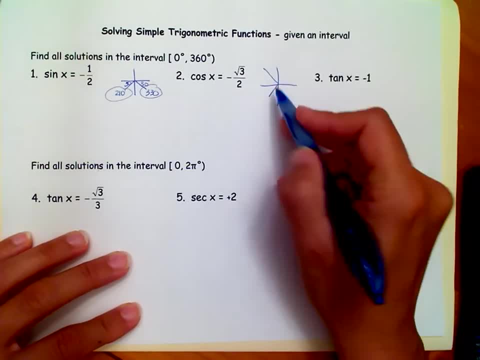 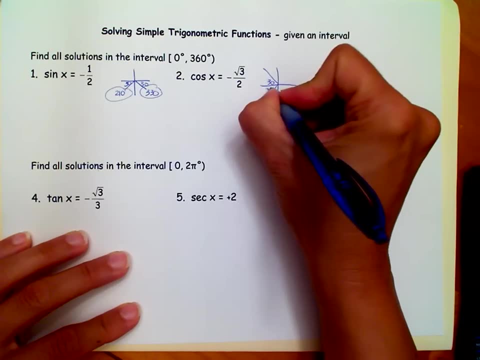 We know that it's going to be negative in these two quadrants, because when you go left on the x-axis, that's when you have it negative. So, since we know that these are going to be 30 and this is 180, we go subtract 30 and add 30.. 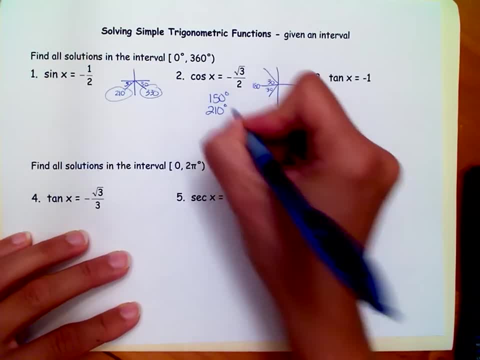 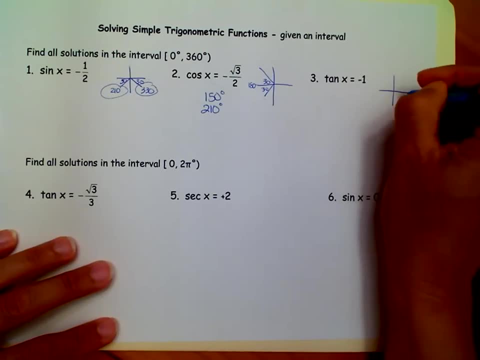 So that's 150 and 210.. Those are our answers there. Okay, when is tangent one Notice? I'm ignoring the negative, initially because I don't have negatives on my chart. So tangent is one at 45 degrees. So now I know I'm at 45 degrees. 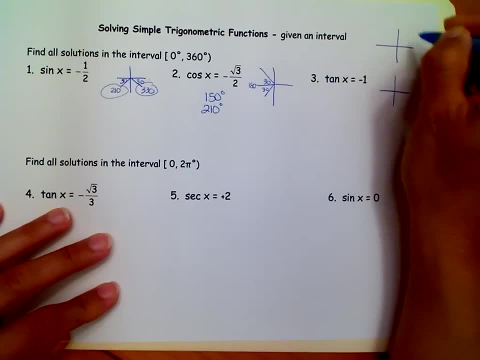 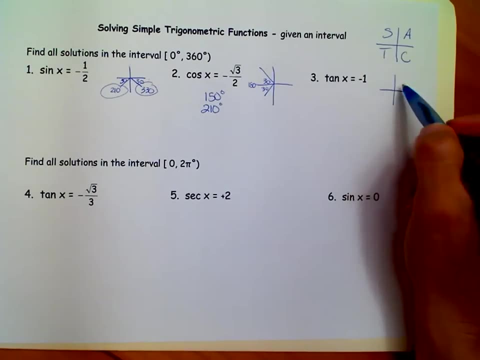 And tangent. well, let me show you this little thing. All students take calculus. That's our little acronym for what's positive and what's negative. So you see, the big plus sign, Those are quadrants. Those separate our quadrants. 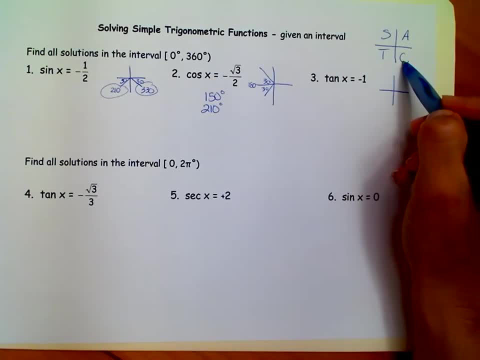 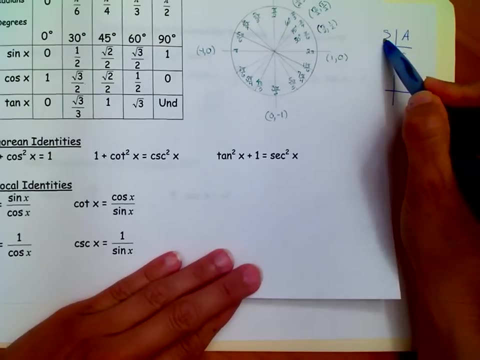 But I just say it's a plus sign, because what this does is tell you where things are positive. All the functions are positive in this first quadrant. Sine and its buddy- remember, sine's buddy- is cosecant. No, I didn't put those on here. 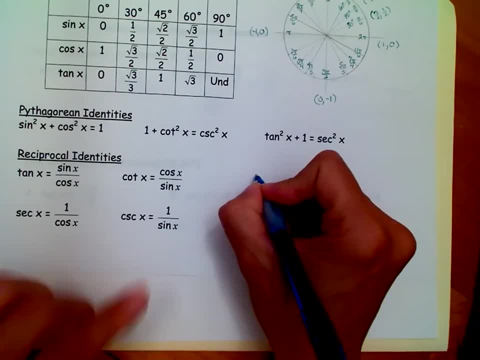 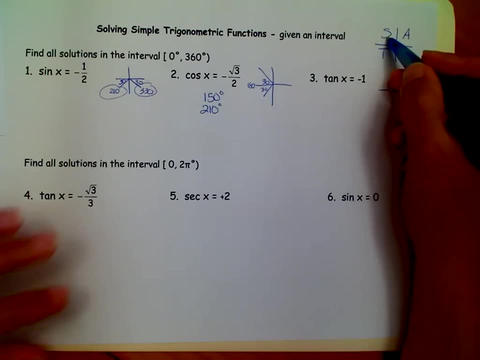 Well, let me do that really quick. Oh yeah, I did Right there. Sine's buddy is cosecant and secant's buddy is cosine, So sine and cosecant are positive here. Tangent and cotangent are positive here. 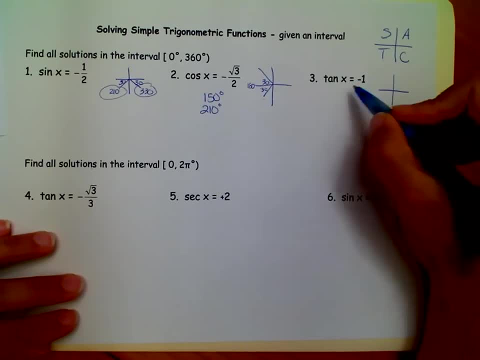 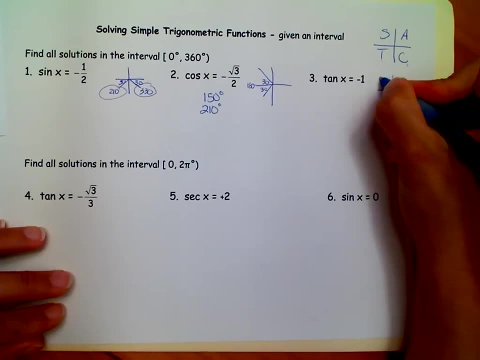 And cosine and secant are positive here. So when is tangent negative? Well, if it's positive here, because everything is positive there and it's positive here, then it's negative in these two quadrants. And since we already noticed that it's at 45 degrees, then we know our reference angle is 45.. 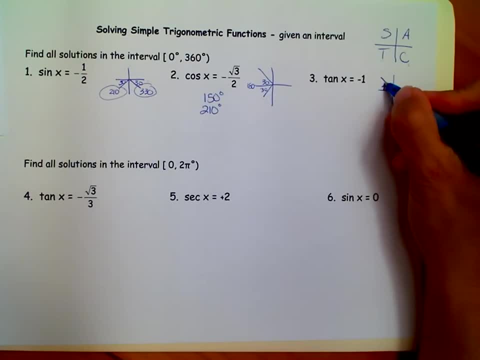 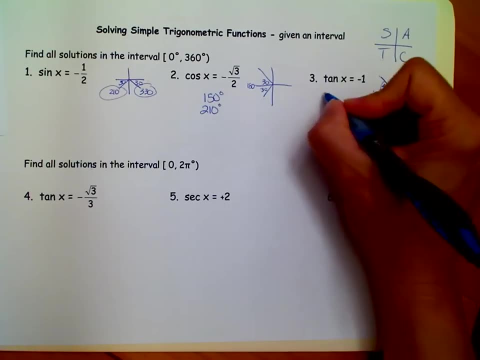 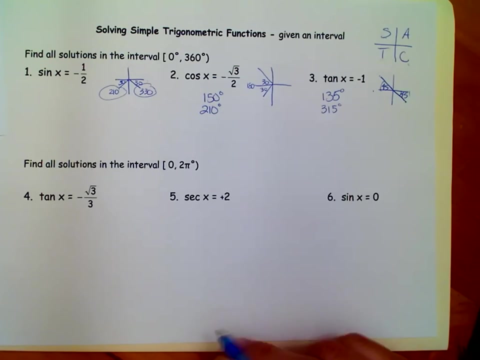 So our reference angle is 45 degrees. here, Remember, reference angles always are how long it takes to get to the x-axis from your line. So 180 minus 45 is 135.. And 360 minus 45 is 315.. So our two answers there are 135 and 315.. 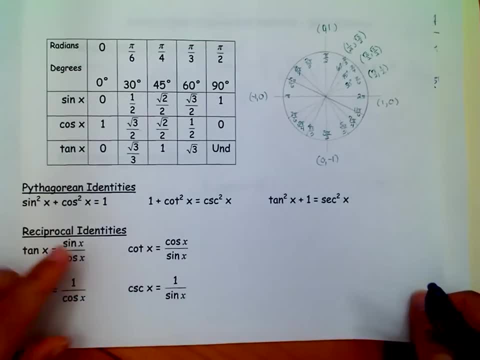 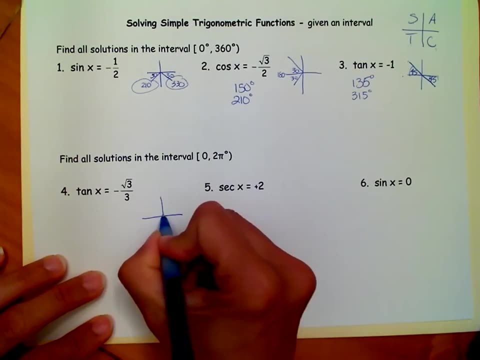 Okay, next one: When is tangent square root of 3 over 3 at 30 degrees? So again, we already decided when it was negative. It's in these two quadrants. So we have our 30 here and here, So we take 180 and minus 30.. 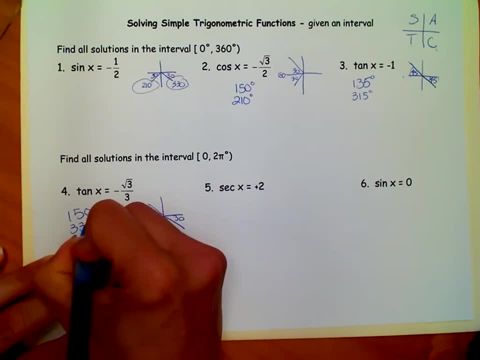 So we get 150.. And then we take 360 and minus 30. And we get 330.. Oops, I'm so sorry, I did not read directions. Okay, so let's change this to pi over 6. And this would be 6, pi over 6.. 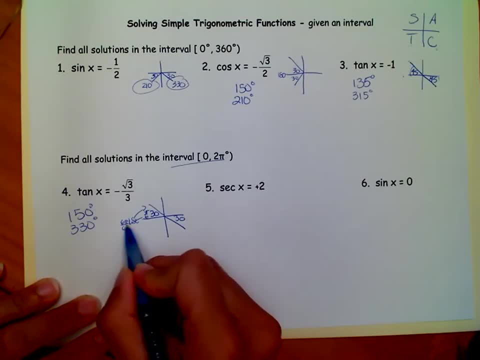 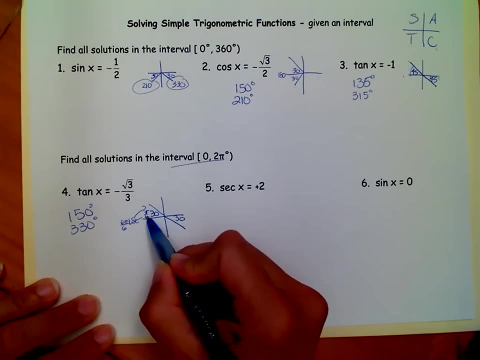 I like to, instead of just saying pi when I'm dealing with pi over 6, to put 6 over 6.. Well, 6 over 6 is 1, but it just helps, Because if 6 over 6 is here and we have to subtract 1 over 6,, then that leaves me 5 over 6.. 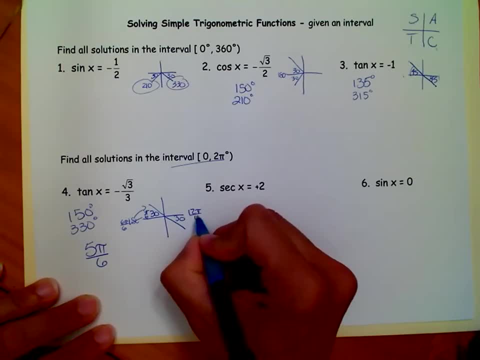 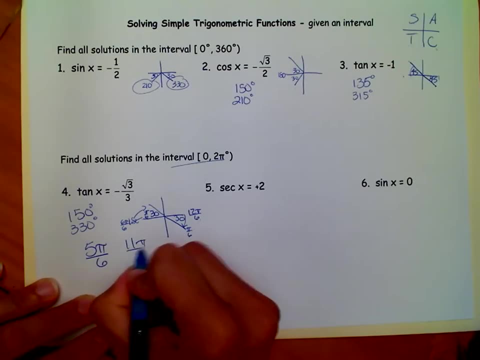 And same thing here. If this is 12 pi over 6,, which is 2 pi- and I know I have to subtract or go down pi over 6,, then I know I'm at 11 pi over 6.. So those are the two answers, which are the same as these, but just in radians, because they asked us to do it in radians. 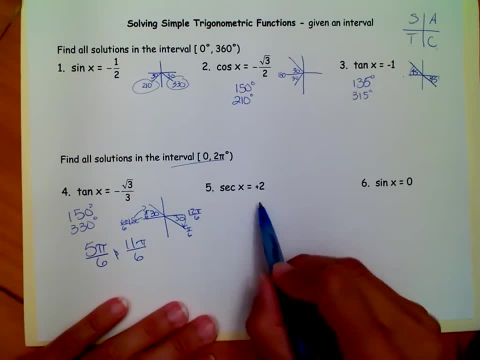 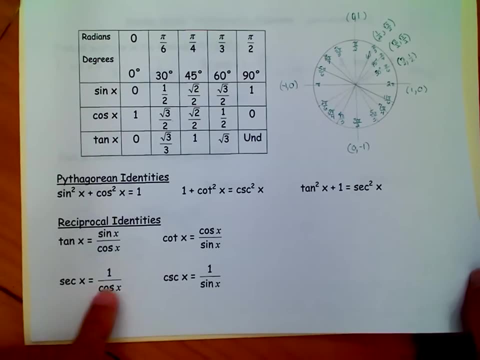 So I changed this to positive because I noticed that there were a lot of negatives. So we need to know when secant is positive, 2.. Well, remember, secant is the reciprocal of cosine. So I want to know which one of these flipped over would be 2.. 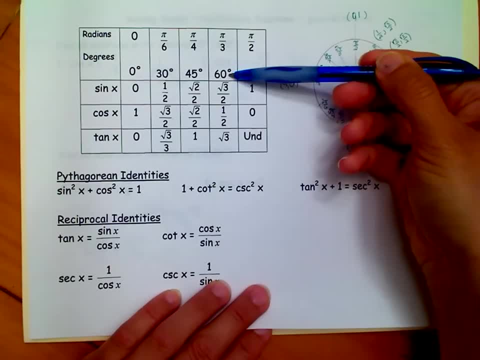 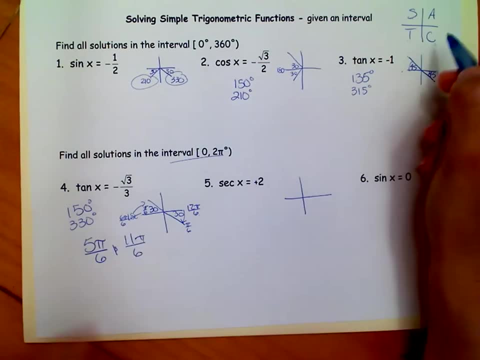 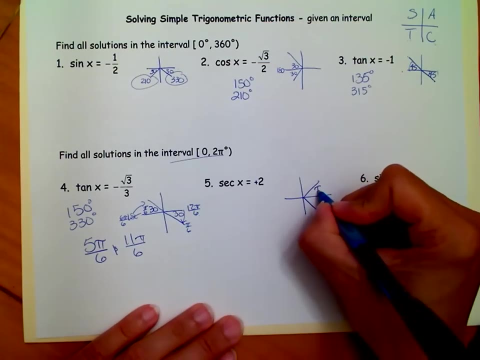 That's this one. So I know I'm at a 60-degree reference angle. So, dealing with cosine, remember, cosine and secant are positive here and here, And I know I'm at a 60-degree reference angle, Or a pi over 3.. 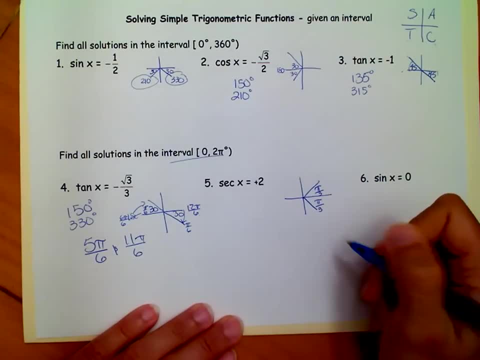 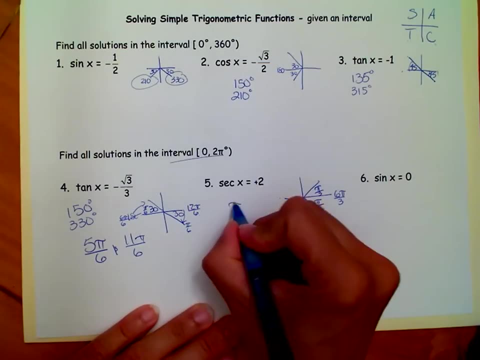 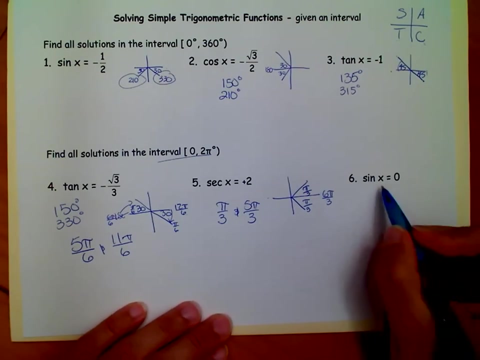 That's the radian version of 60. So this is 3 pi over 3.. This is 6 pi over 3.. So I know I'm at pi over 3 and 5 pi over 3.. Okay, When is sine 0?? 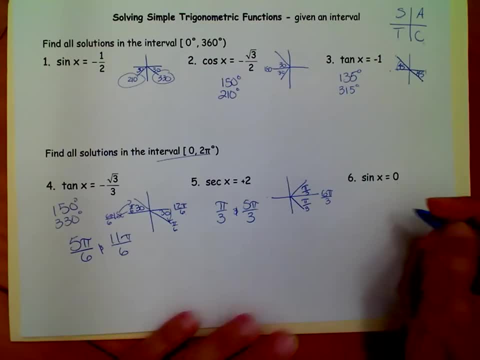 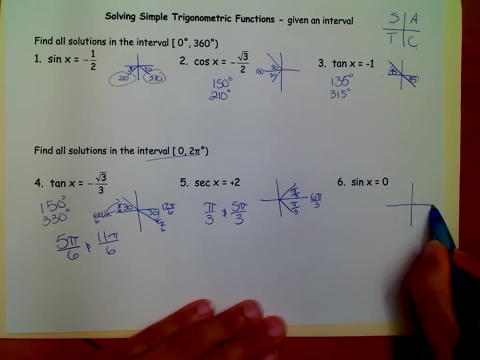 Last one: Sine is 0 at 0. Where else? Well, when sine is 0, that means sine is y. So I'm not up and I'm not down. I would have to be straight right or straight left. 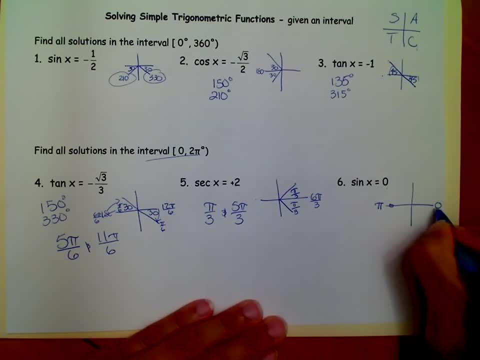 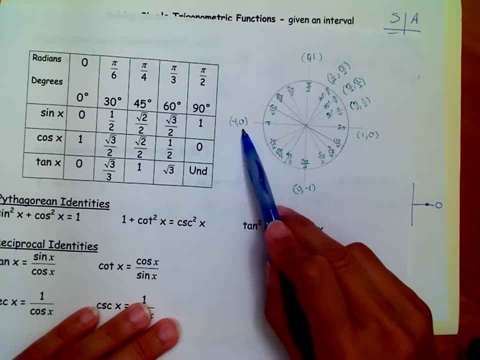 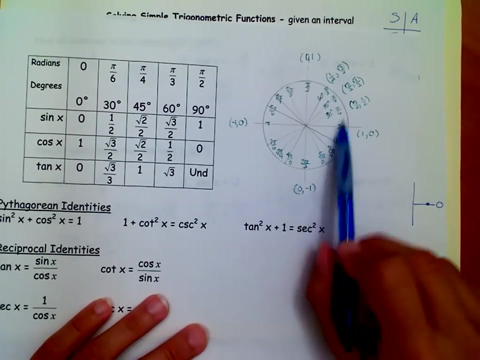 So that's at 0 and pi And you can see on this little chart: remember, sine is y And y is 0. here and here- And the book has, almost every book has one of these little charts, maybe in the reference section, in the back or in the front flap.